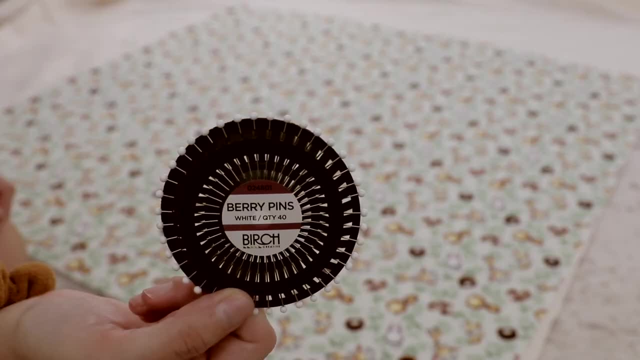 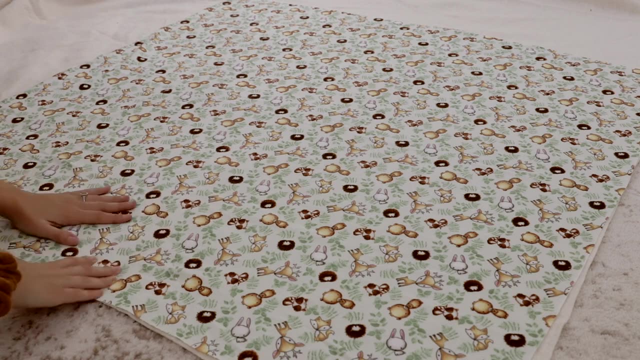 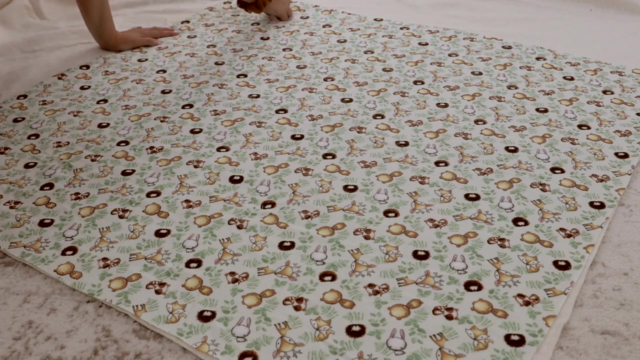 down on top of that with the right side facing up. I then just took some pins and pinned all over the fabric to hold the wadding to the flannelette. I do recommend using safety pins over pins. if you don't have safety pins, you're just less likely to prick your finger or anything like that while you're sewing. 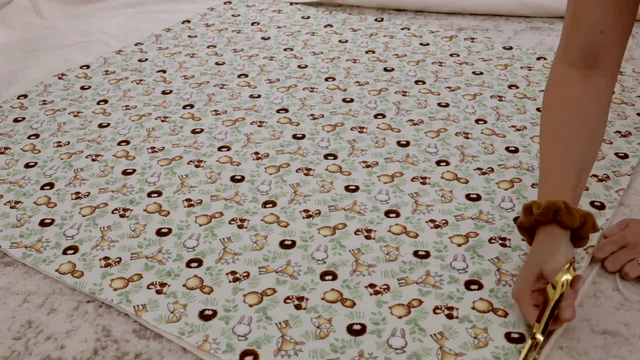 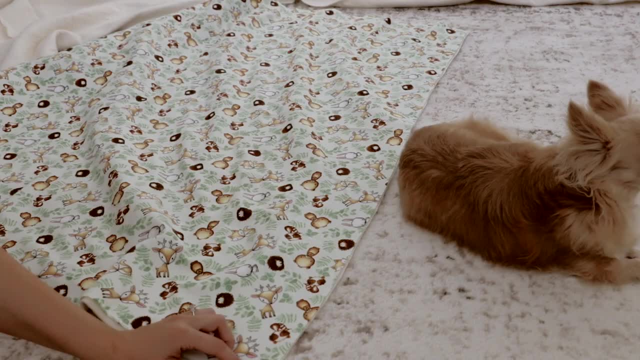 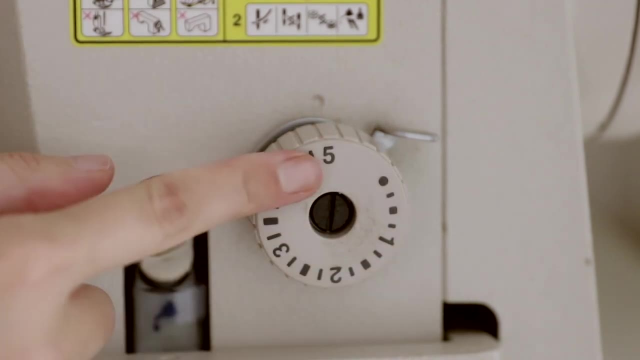 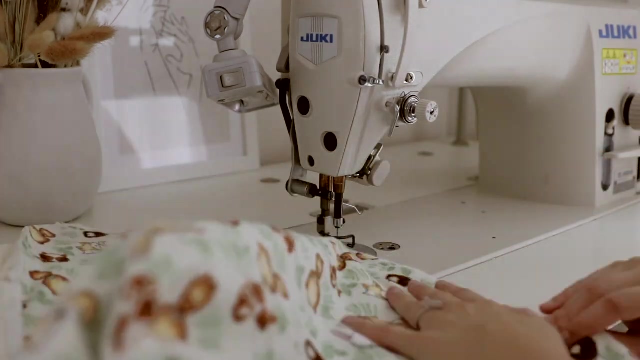 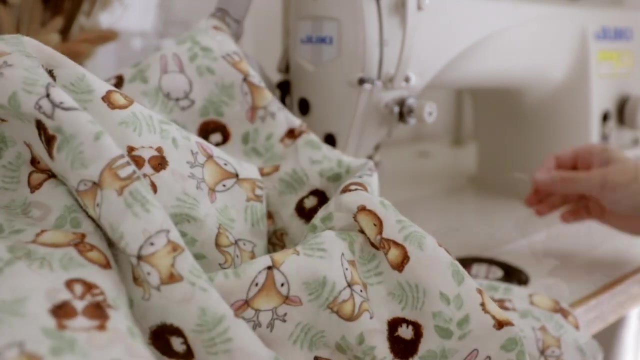 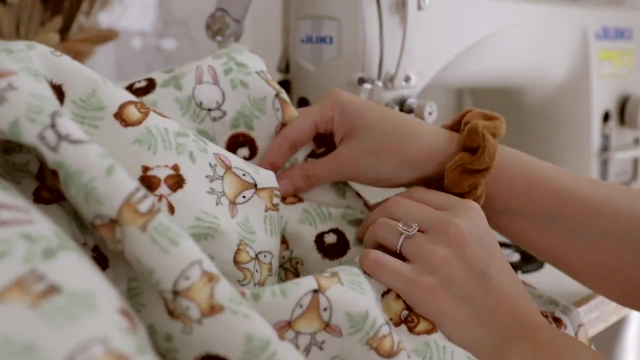 Once that was all pinned down, I then cut the wadding to the same size as the flannelette. I then did a basting stitch around the entire edge just to hold the flannelette to the wadding. Doing that, I pick up a pair of swagt新聞 pins and the fidget spinners and pin stitches and the waterón. Boobs and scissors and then pull the end out onto a flat white fabric pad. Once I had finished basting the entire thing, I then took all the pins back out. Here I'm laying out the base layer of the playmat. so if I'm using a mattress bra. 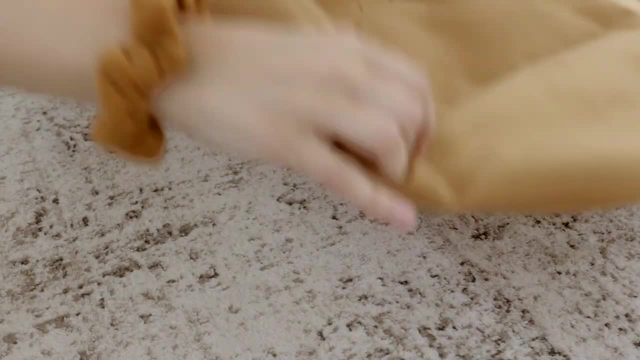 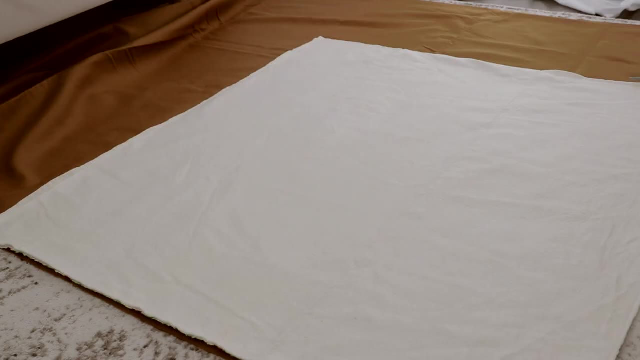 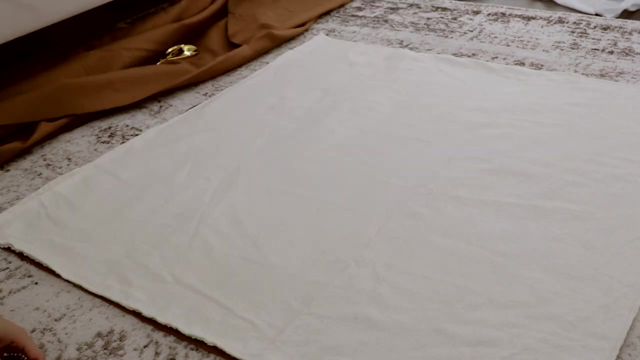 you're making this as well. make sure that your right side of the fabric is facing up and then place the right side of the flannelette fabric facing down onto the base layer. next i'm pinning all of the edges so that i can sew it together. i'm also going to leave a gap to. 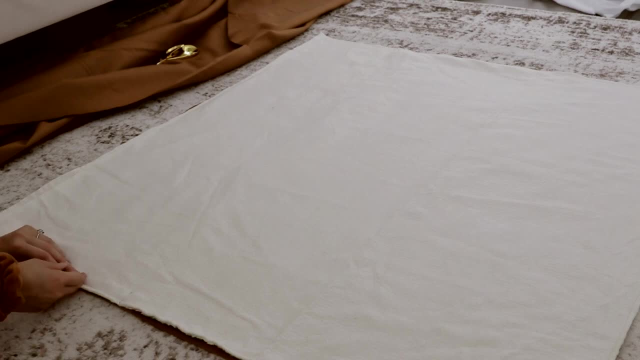 turn it inside out. if you do make this, i recommend leaving the gap a little bit bigger than i did, because the fabrics were quite thick, it was a little bit harder to turn inside out. i also like to pop in a pin horizontally, so i remember not to sew in that section. 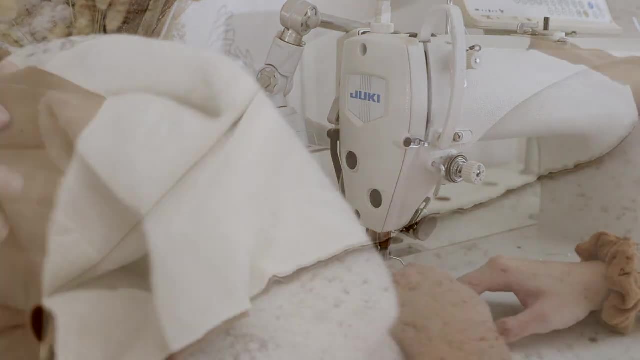 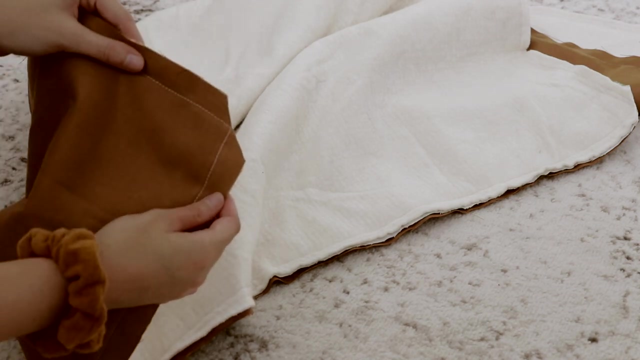 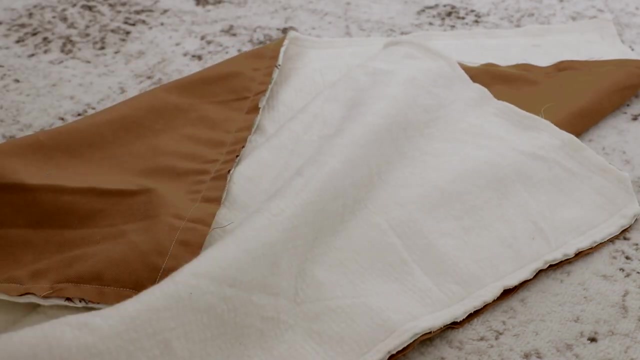 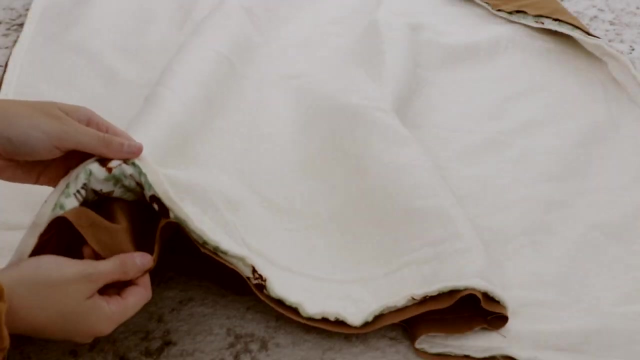 once i had finished sewing the edges, i then went around to each corner and snipped it off like this. this just gives you a sharper corner when you turn it inside out. when turning it inside out, i found it easiest to feed my hand into the top corner and then. 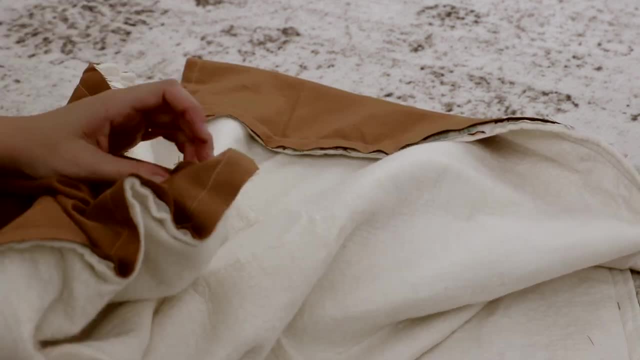 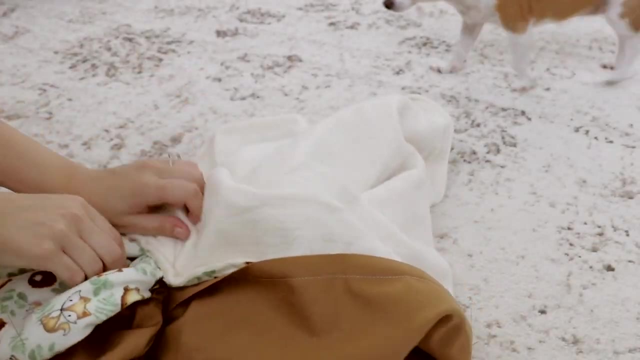 i'm just going to turn it inside out like this. so i'm just going to turn it inside out like this and then pull that through first and then work by pulling each corner out. and because i was filming on the floor, charlotte thought that it was playtime, so she came over for a little kiss. 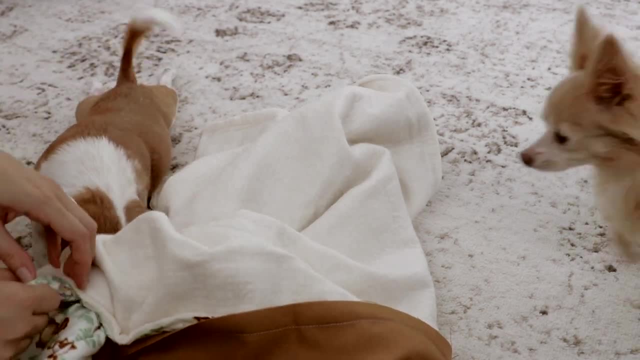 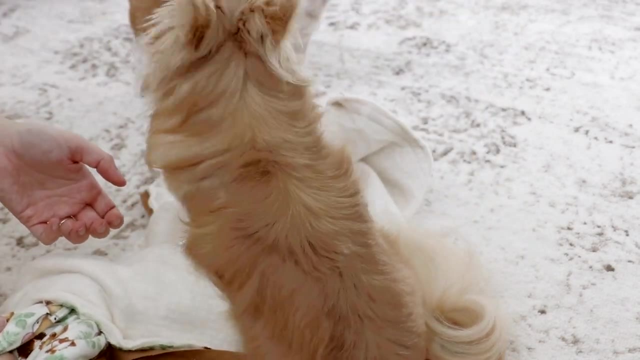 and cuddle. and then, of course, moon thought that i was making this playmat for him, so he wanted to sit on it the whole time and i had a bit of trouble kicking him off. i think i'm going to have to make him his own special playmat. what do you guys think? 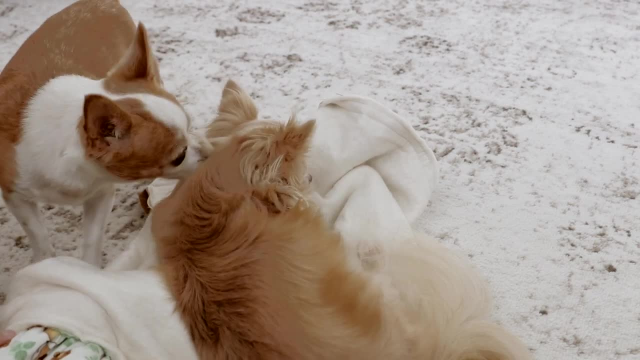 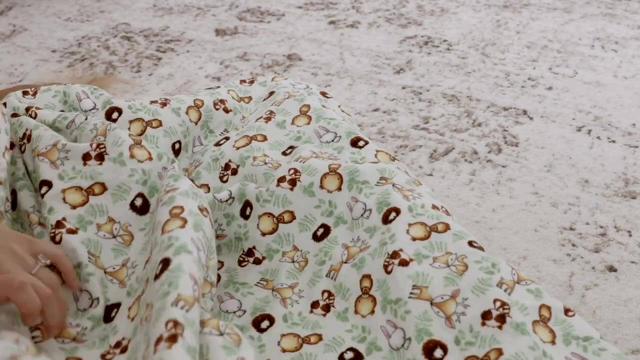 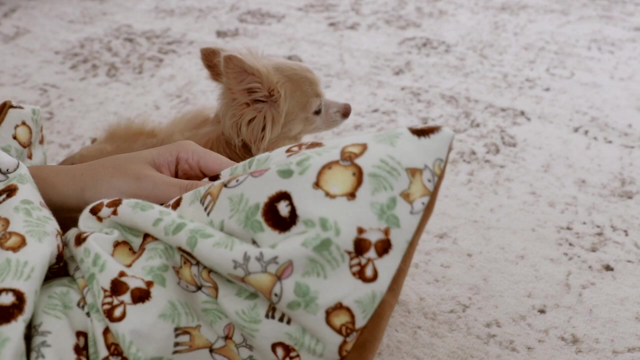 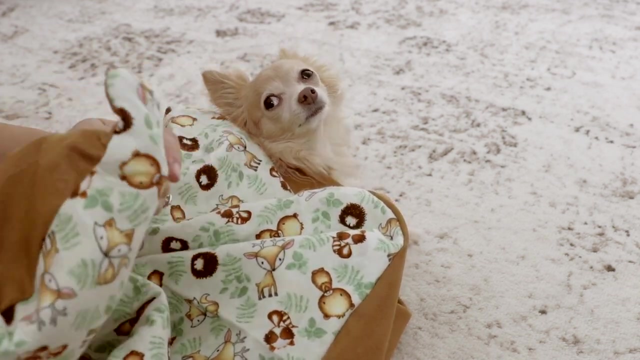 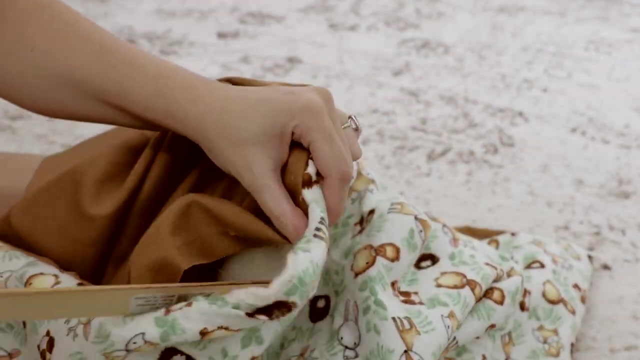 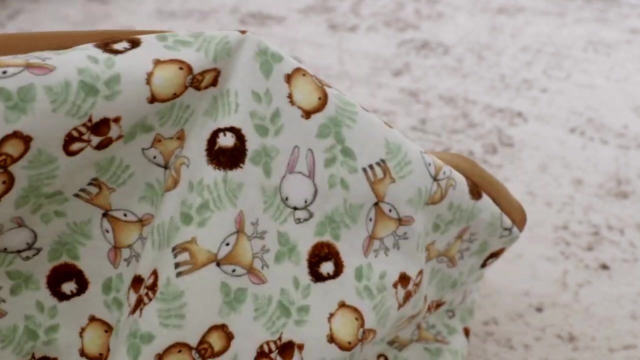 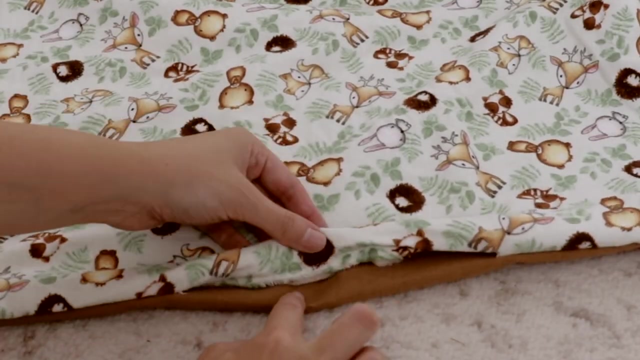 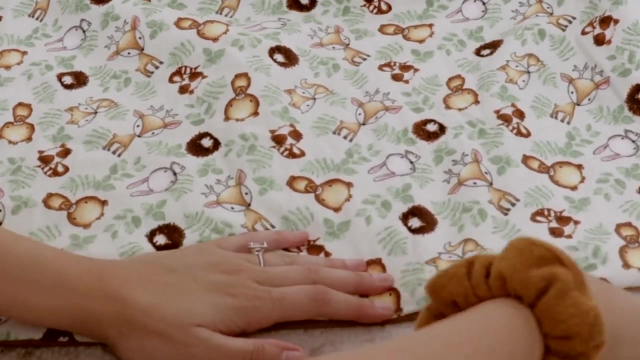 so so. so Once I had completely turned it inside out, I then grabbed a ruler and ran it along all the inside edges just to press the seam out. This works well to push your corners out as well, Moving on to the opening. so I just made sure my seam allowance was tucked in neatly and then I pinned it down ready to sew. 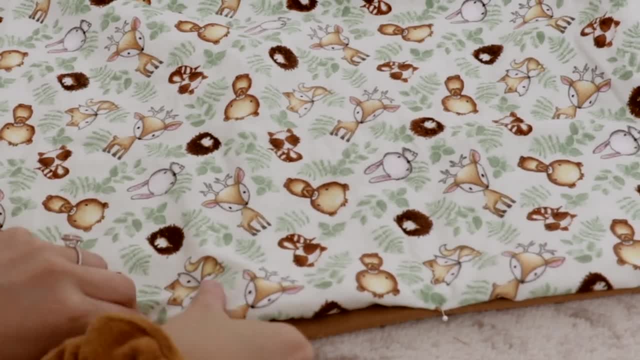 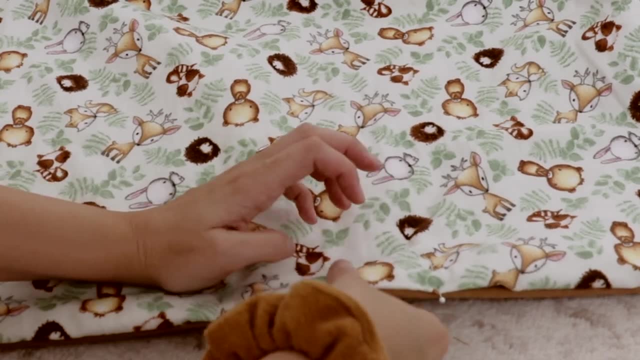 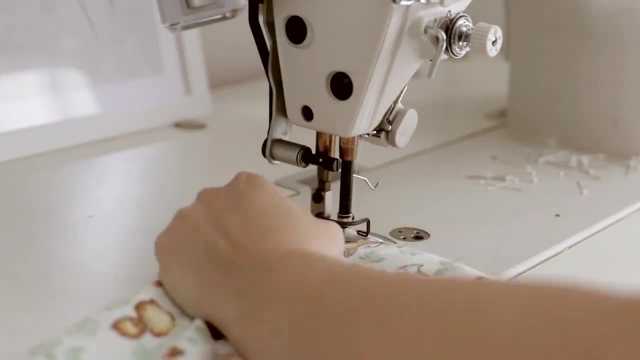 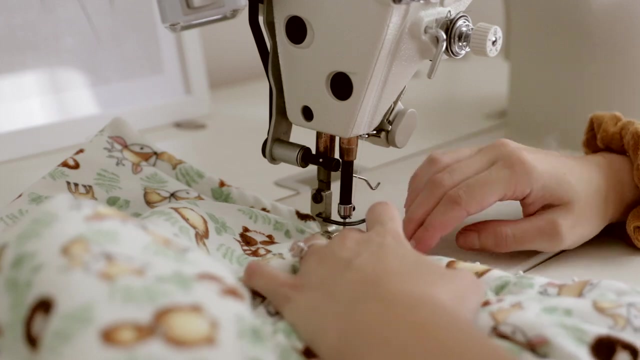 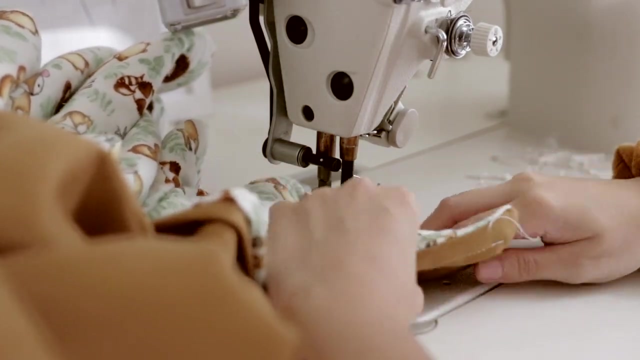 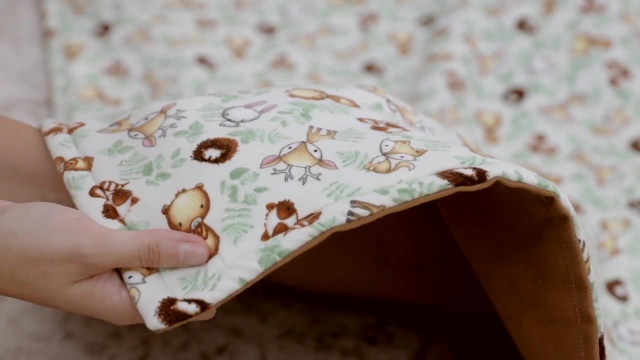 And then, to finish, I sewed a 1.5cm seam allowance, and this also closed that opening that I just pinned together as well. So this is what the finished playmat looks like. it turned out so cute and it's so soft and plush. 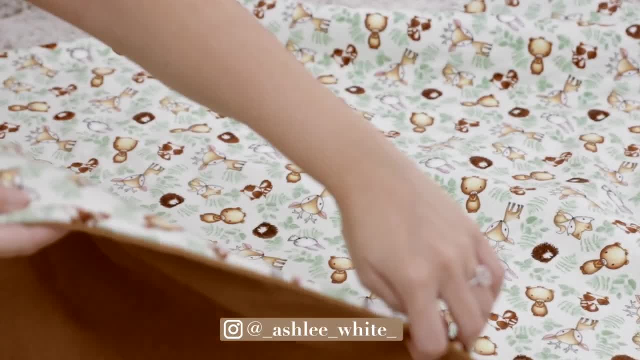 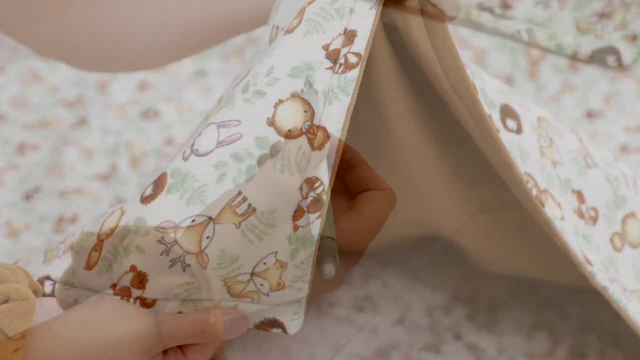 While I was making this, I was sharing it on Instagram, on my stories, and I decided that I wanted to make a little critter to match, and I was tossing up between the little bear and the hedgehog. So I popped up a poll and most of you voted for hedgehog. 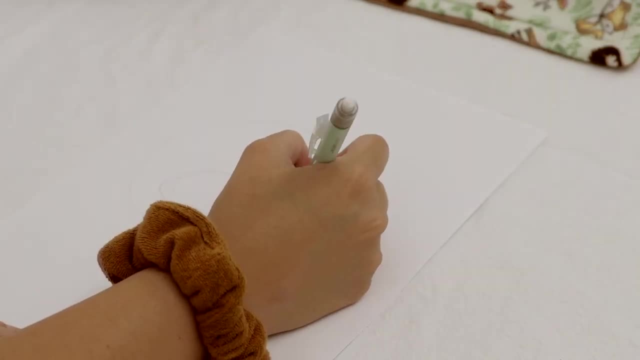 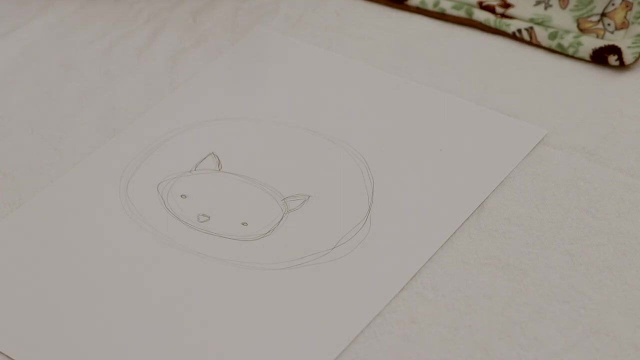 So that's what I ended up making For the hedgehog template. I drew a large circle and then a smaller circle. I originally drew the ears quite pointy and then I realised that hedgehogs have round ears, so I do change that later on. 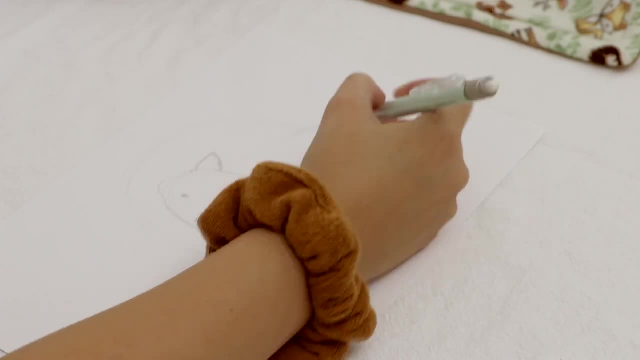 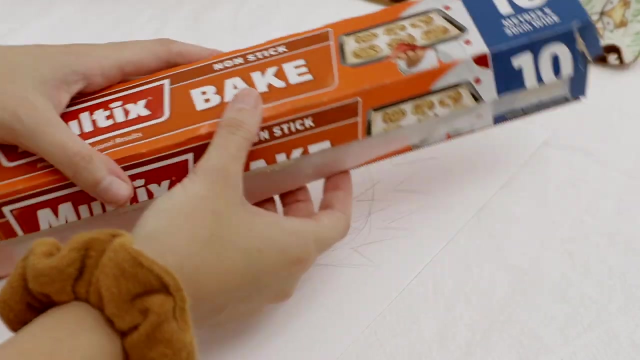 And then here I am, drawing in the little spikes. I do recommend folding your paper in half and drawing it that way. I didn't think about this before I did it, because I did it on a bit of a whim, so there was no planning. 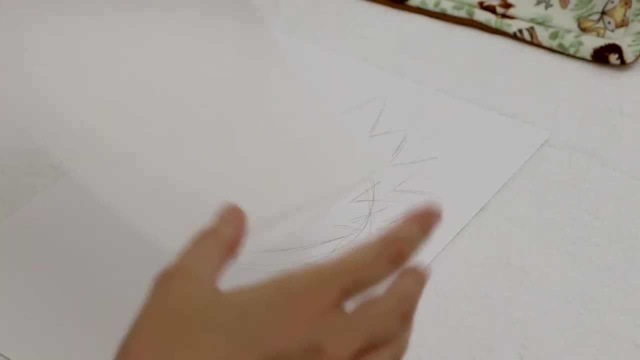 And then I'm taking some baking paper and folding it in half. So I did just go back in and fix the spikes up so that the middle of the spike met the fold of the paper. This just makes it so much easier when you're cutting out the pattern. 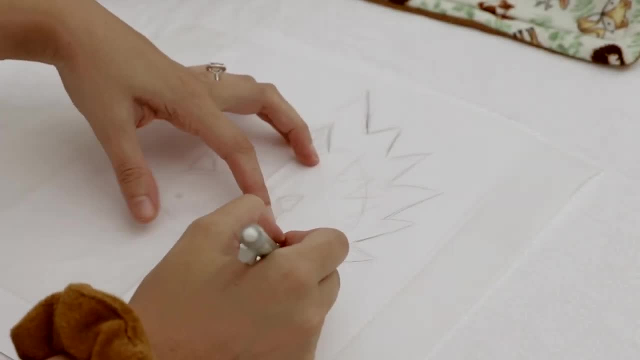 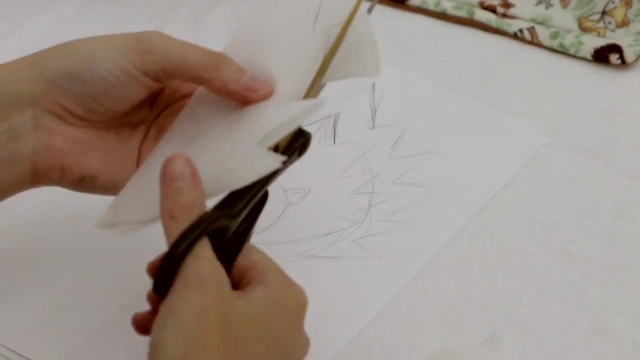 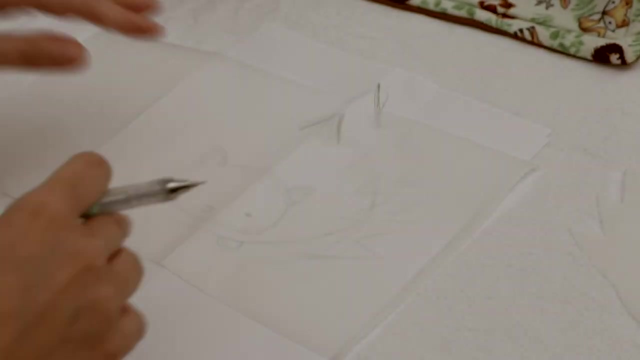 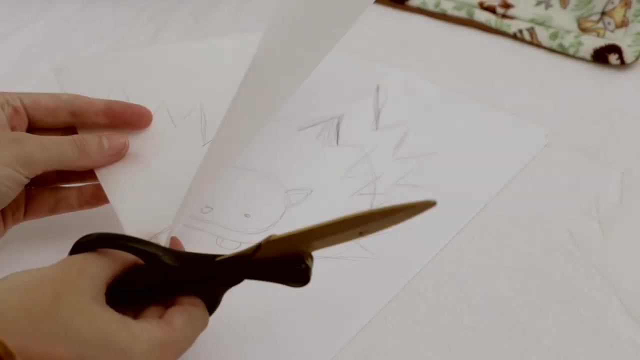 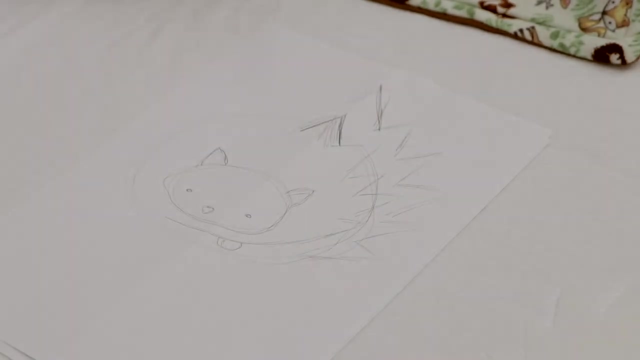 So here I am just tracing over the main part of the body and then folding it in half and cutting it out, And then I've gone ahead and repeated the exact same thing for the smaller section of the hedgehog, And then next I'm tracing the face and redrawing the ears to be more circular, like they're meant to be. 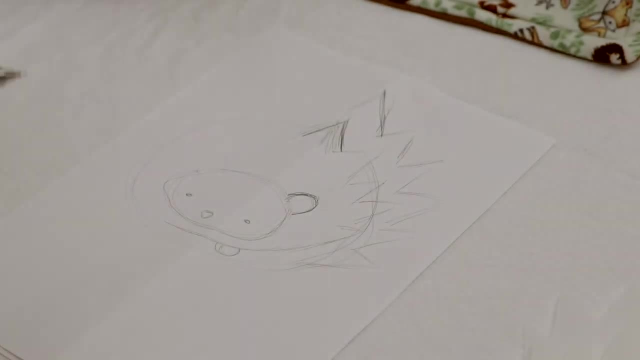 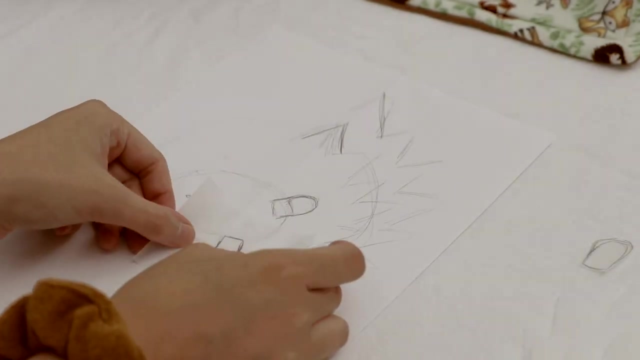 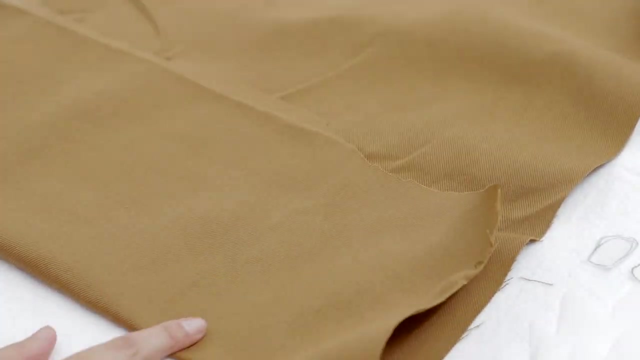 And then, when tracing off the ears, make sure you add some extra seam allowance here, because you want it to tuck behind the face. And then the same for the feet as well. And then for the largest piece of the hedgehog pattern, I cut out two layers, so I've just folded my fabric in half here. 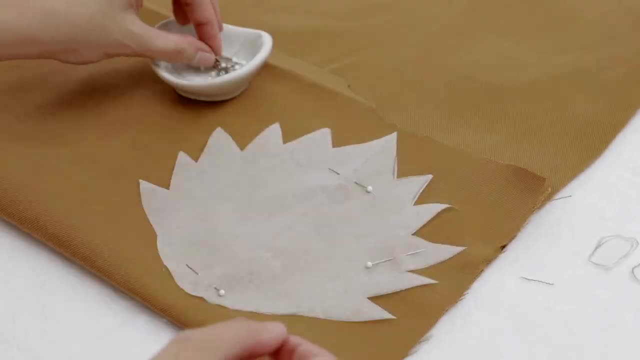 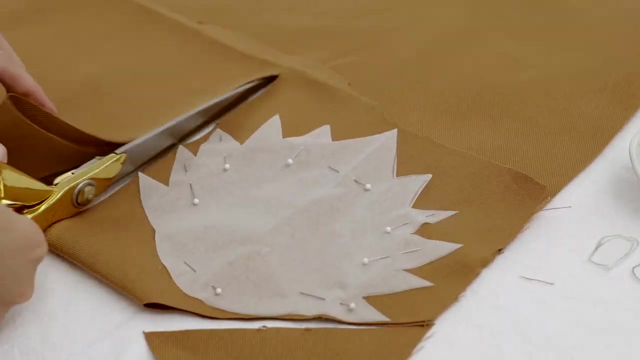 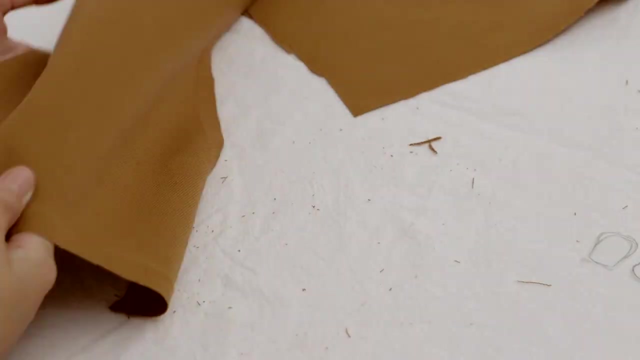 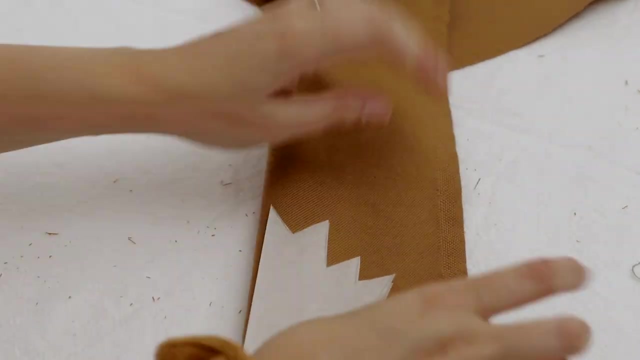 Pinned it down and then cut it out, And then for the smaller body piece I only need to cut out one piece. I realised that when I went to cut out the fabric, So I've just folded that in half to save on cutting time and pinned it to it. 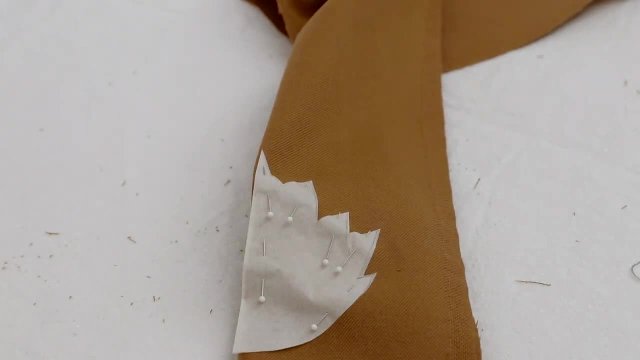 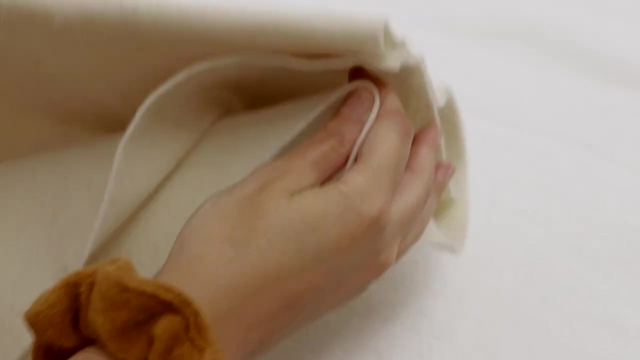 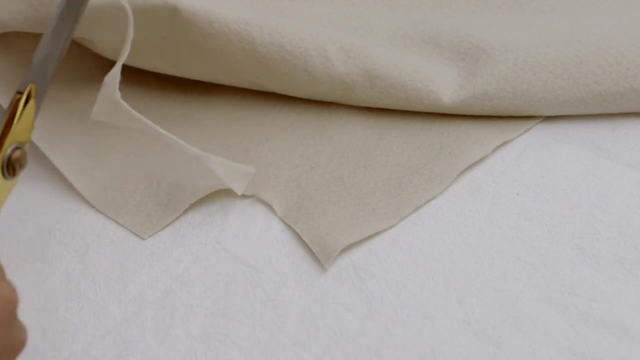 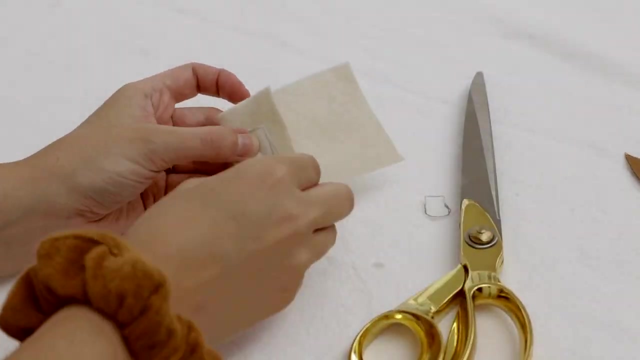 And then I made a folded piece of fabric For the face, feet and ears. I ended up using this cream felt. I've just sped this up, So you just cut out one of the face, two of the feet and two of the ears. 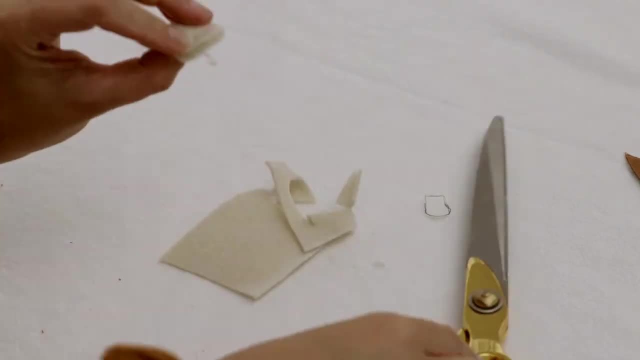 For the face. I ended up, using this cream, felt and cut the areas. this is really easy and easy to work with. Look at the movement here. the face: I decided to stitch it in, so I've just created a little triangle for the nose. 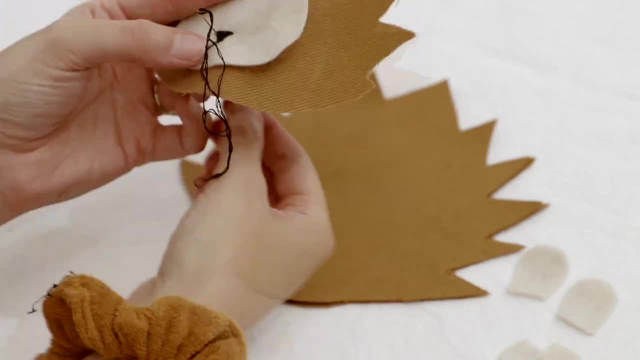 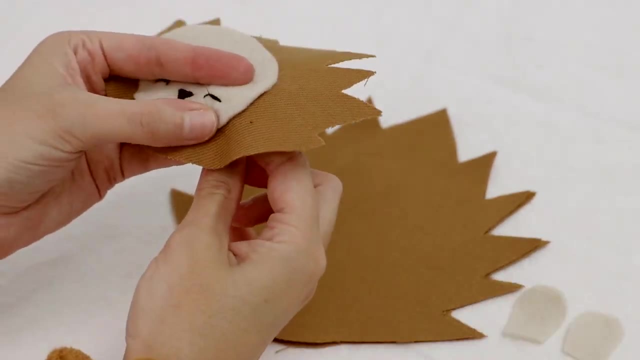 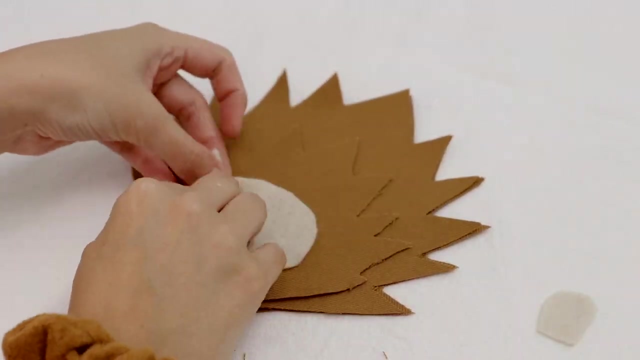 and then I worked my way back and forth to fill it in, and for the eyes I did a straight line and then two little angled lines off to each side and I just went over until I was happy with the thickness of the thread. For the ears I folded them in half and then pinned them down. I also 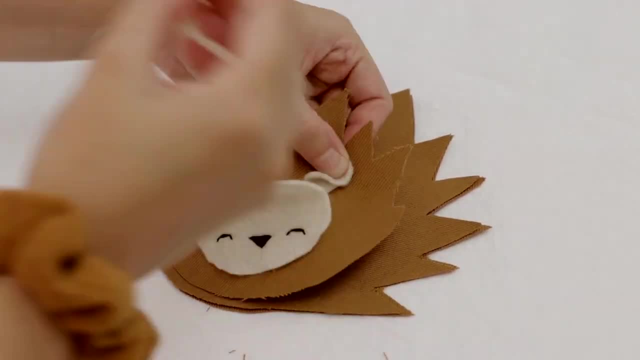 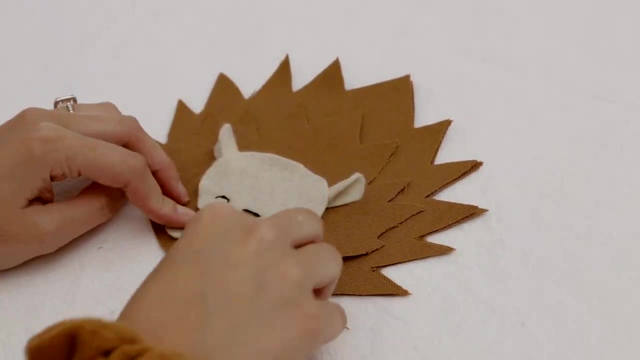 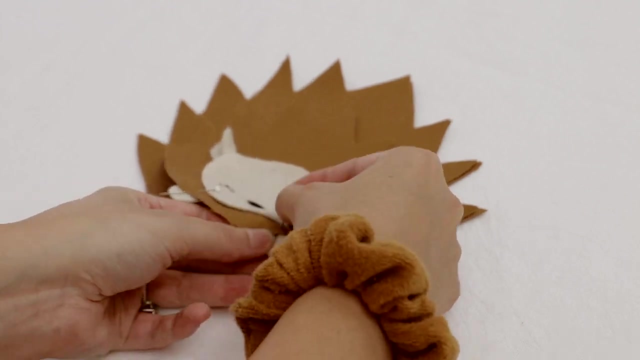 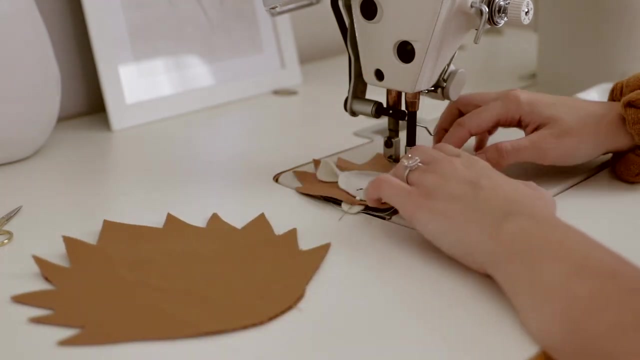 popped in a few stitches to hold them in place until I sewed the face on, and then I also positioned where I wanted the little feet to go To assemble the hedgehog. I started by sewing the face down and I probably left about a five millimeter seam allowance. 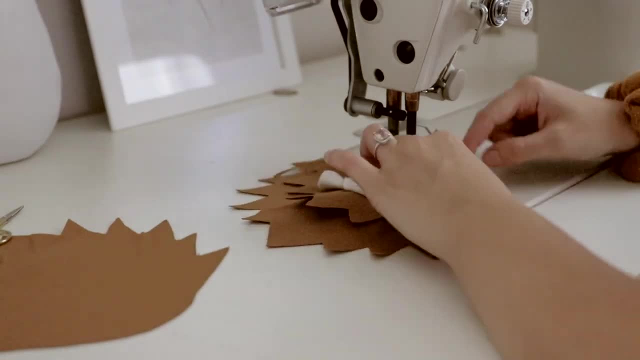 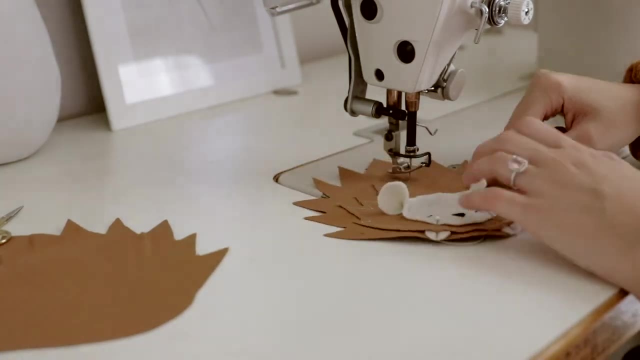 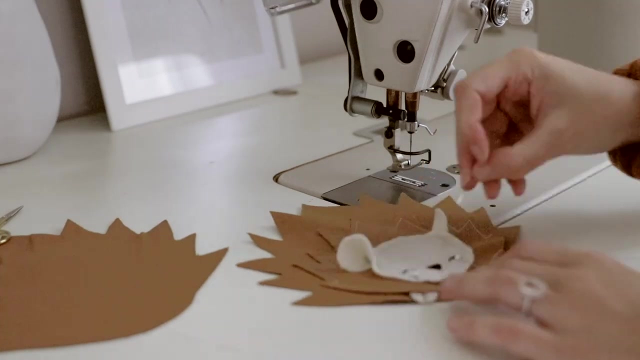 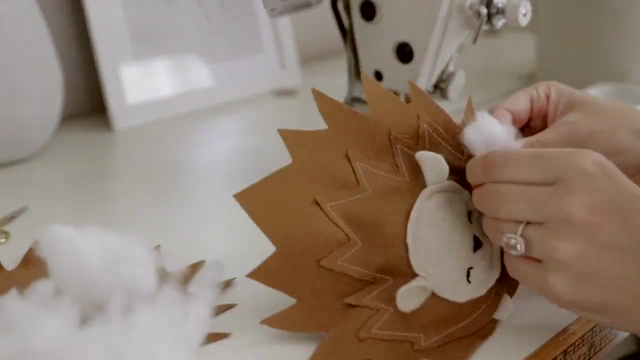 And then I attached the smaller section to half of the larger section of the hedgehog and I left a small gap to pop some stuffing in here. So for the stuffing I usually just buy the two pack of pillows from Kmart for $5.. You get lots. 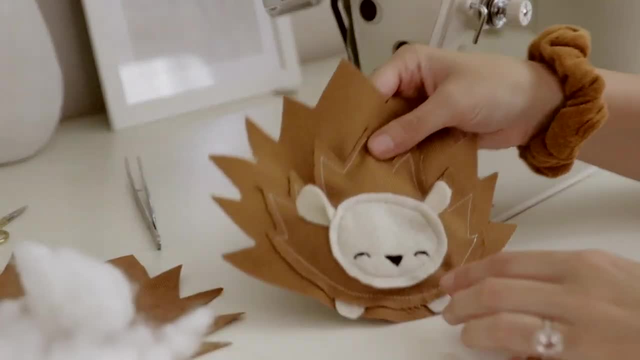 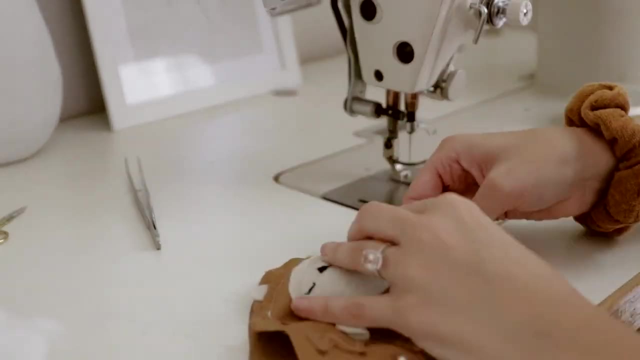 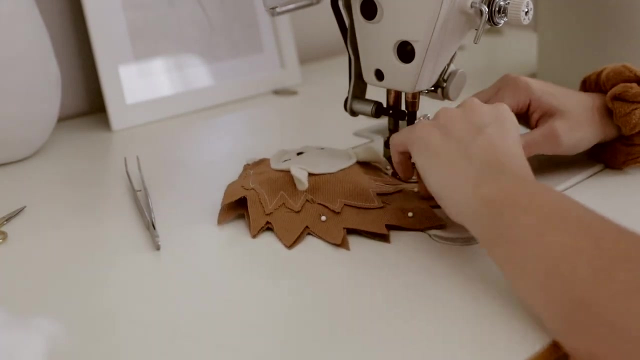 of stuffing And then I'll fill whatever you'd like to call it. It's very affordable. So I've just filled in that front piece and then stitched it closed, and now I'm attaching the two large pieces together and again leaving a little opening to fill it with stuffing. and then, once I'm done with that, I